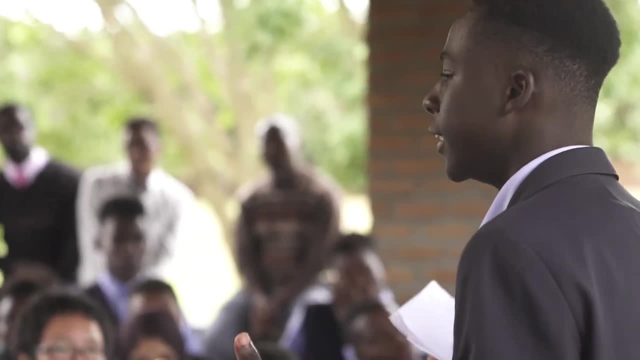 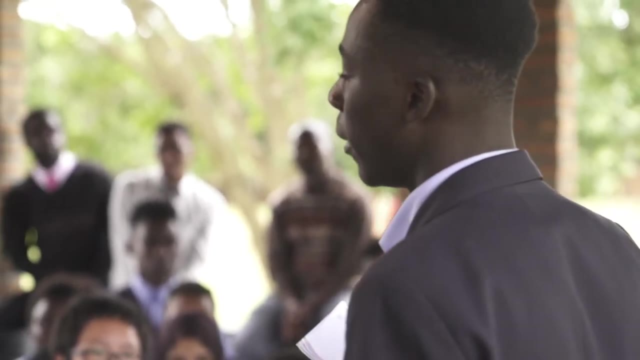 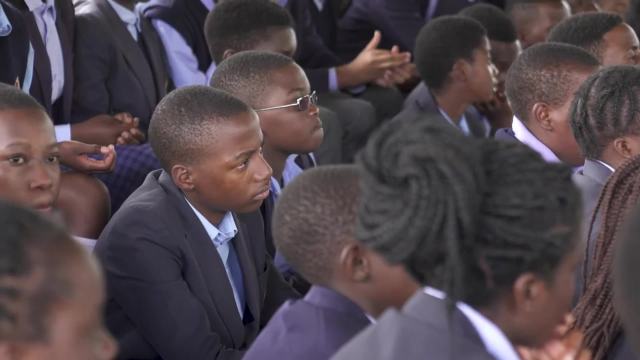 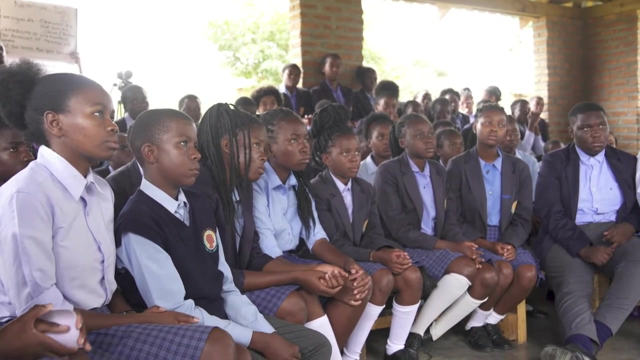 With colonialism, democracy came, We took over. But the sad thing is that democracy came in with dictatorship, But with the referendum. the referendum challenged democracy, The referendum challenged dictatorship. Later on, here we are practicing this democracy, We are enjoying this type of ruling. 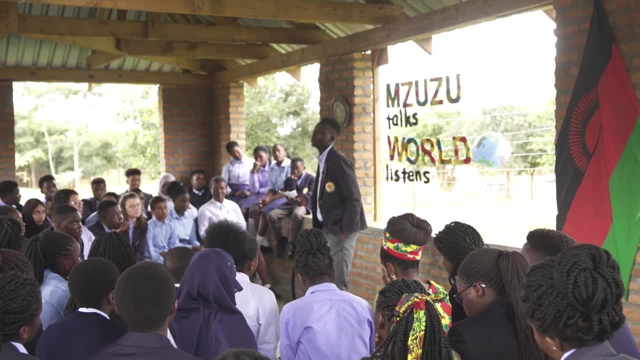 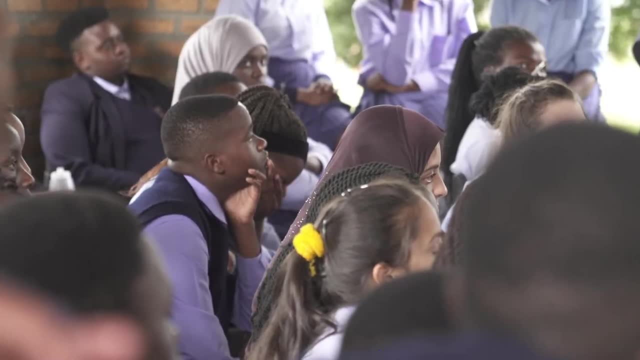 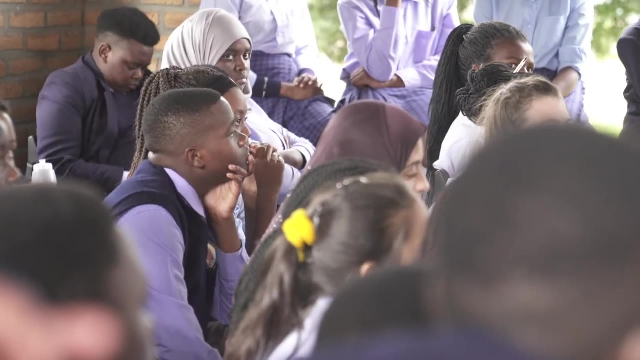 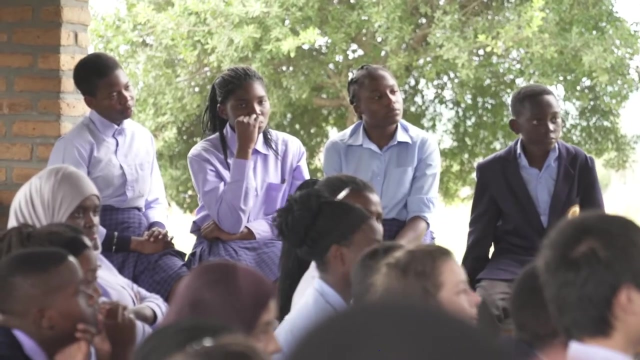 But this type of democracy is broken. You may ask: what do you mean? This type of democracy is corrupted, People are corrupted, We have irresponsible students, We have irresponsible citizens here right now. And what you need to know, you have the responsibility. 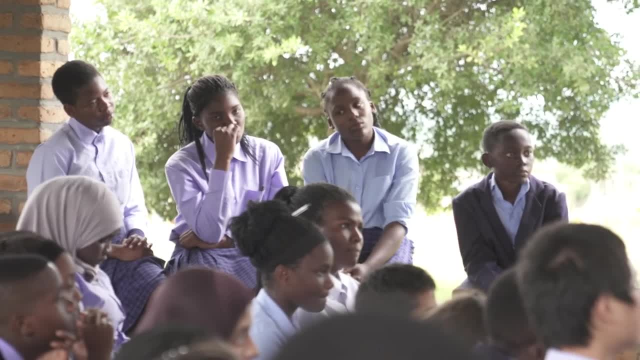 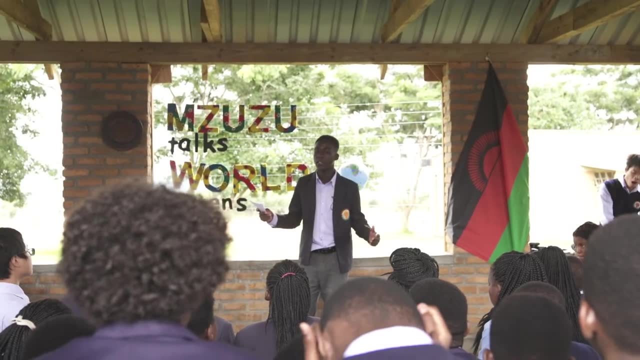 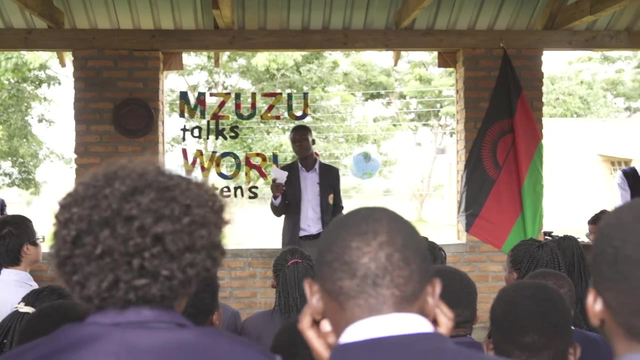 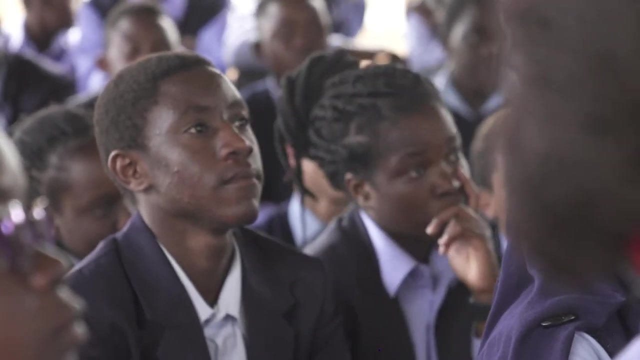 We have a lot of people here in Malawi. We have people who are supposed to vote. Unfortunately, sadly, those people are not even registered. It's only 5.4% of people here in Malawi who are registered And we are supposed to choose the right leaders. 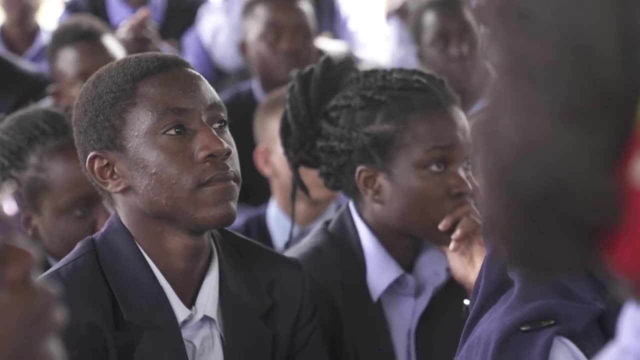 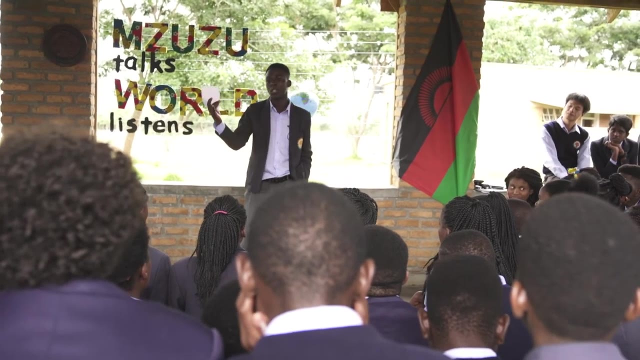 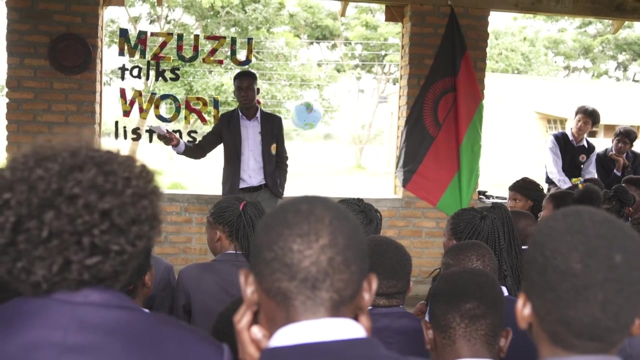 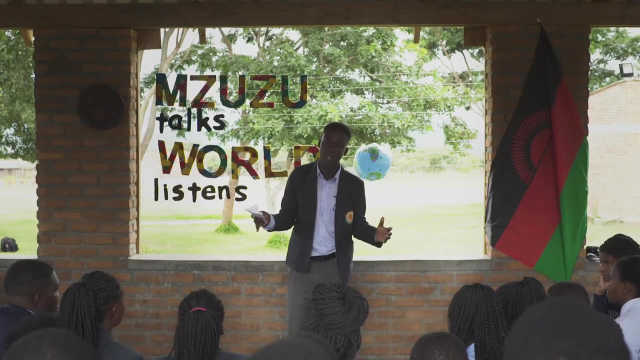 We have problems. Corruption, We have problems. You have been talking about child marriages. All this because of our poor leadership, Because our leadership is poor And the power is in your hands To choose the right leaders, But the foundation of these problems is that we are limited to knowledge. 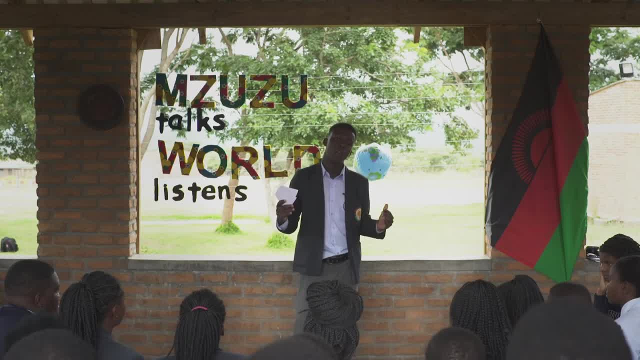 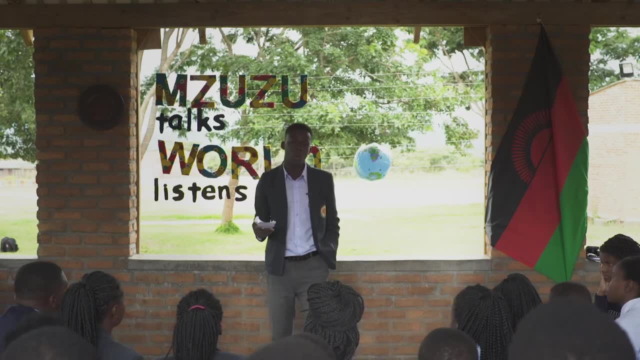 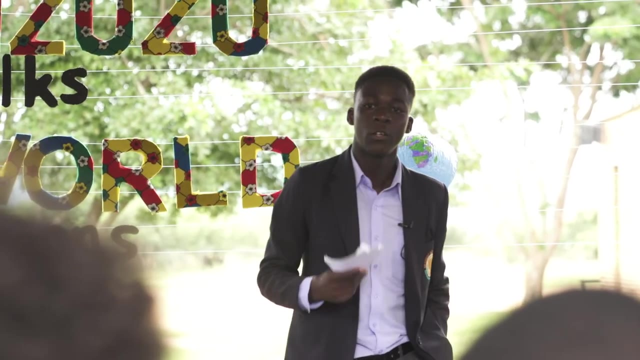 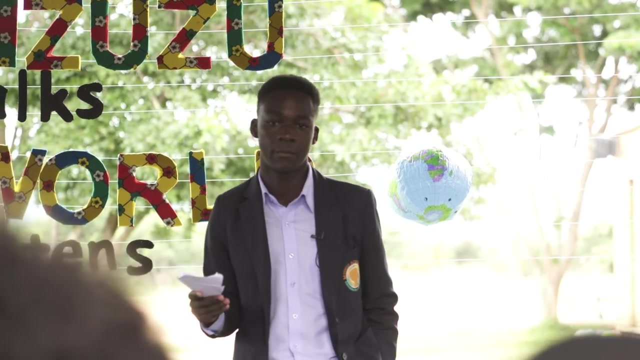 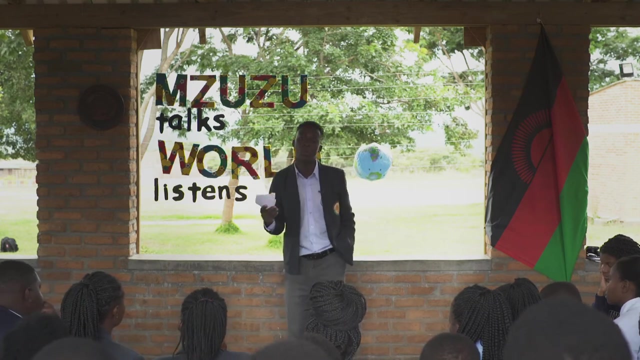 Limitation of knowledge of values and principles of democracy. Related to that is that we lack- We lack dissemination of information, which we are supposed to have to achieve necessary and accountable and transparent system of government. However, we can be talking about all these problems.